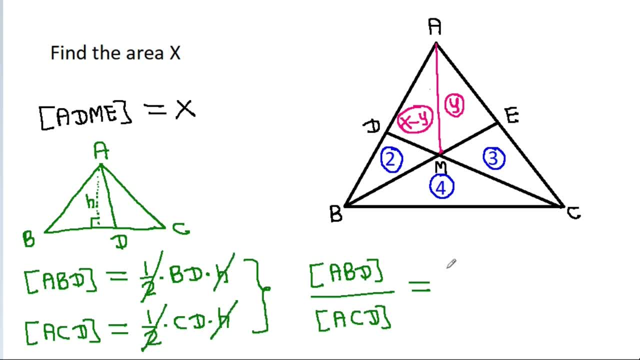 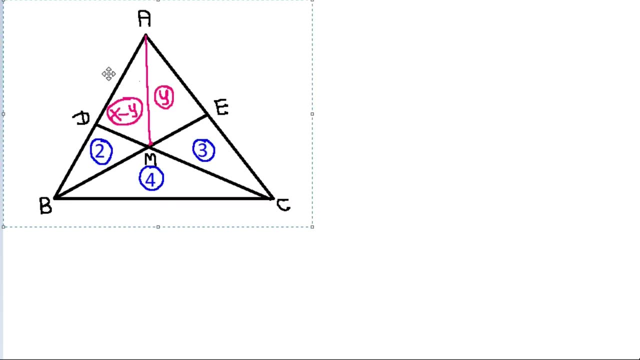 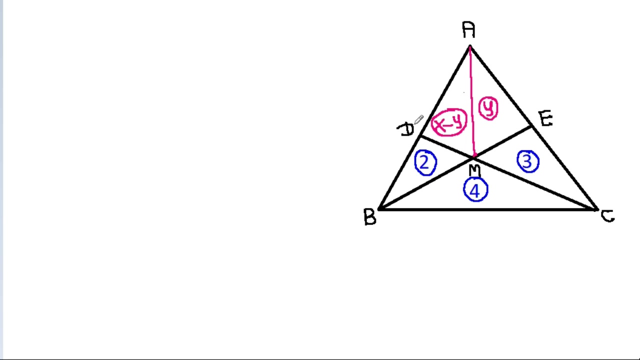 and H will get cancelled, So it will be BD by CD and BD by CD. Suppose AD is A and BD is B, Then it is A, B and M And this point is D and AD is A, BD is B and this area is 2 and this area is x minus y. 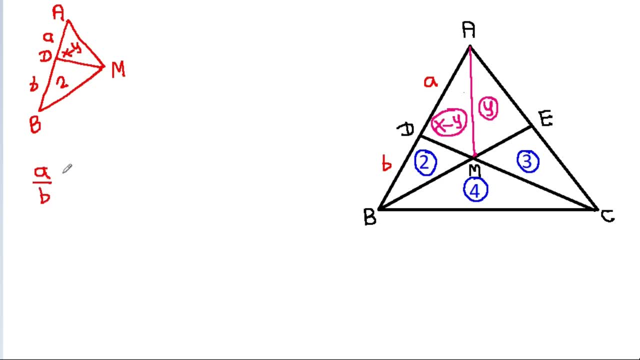 A by B, it will be equal to, And also in A, A, B, C, and this is D, AD is A, BD is B, and this area it is X minus Y, minus Y minus 3, that will be X minus 3, and this area it will be 2, minus 4,, that will be 6.. So A by B. 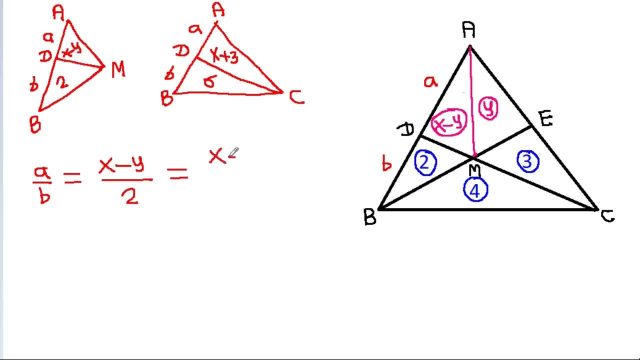 it will be also equal to X minus 3, by 6.. And from this equation, if we cross multiply, then 6 times X minus Y, it will be equal to 2 times X plus 3, and it is 6 X minus 6. Y is equal to 2 X. 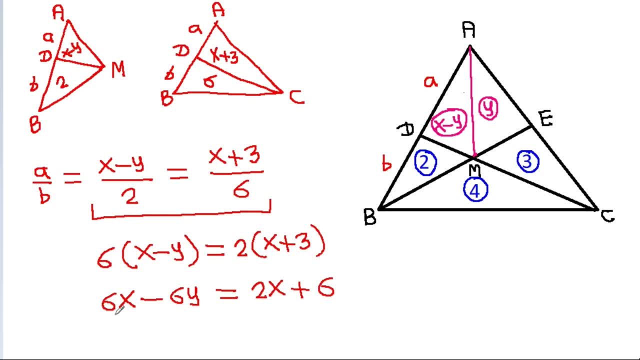 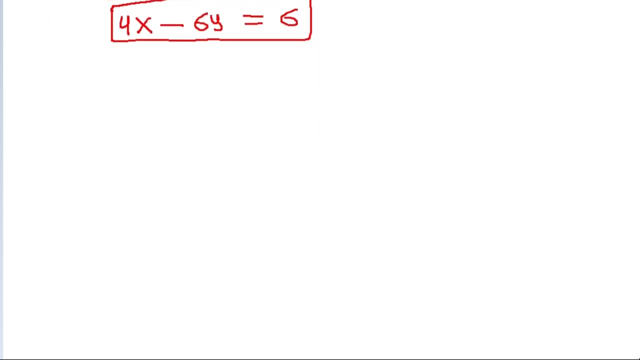 plus 6, and 6 X minus 2 X will be 4 X minus 6 Y, it is equal to 6.. We have A Now. suppose BM is C and EM is D, Then it is BE and A, and this point is M. 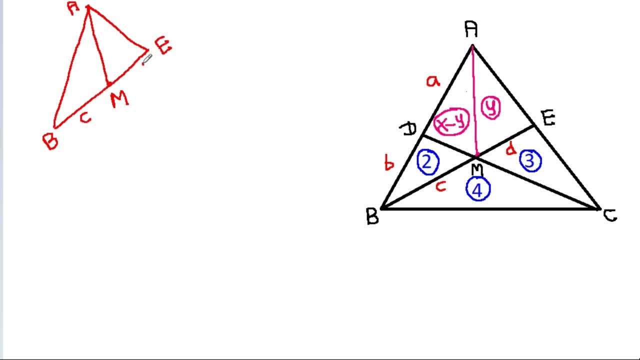 We have BM is C and EM is D and this area is Y and this area it is X minus Y. and this area it is X minus Y, and this area it is X minus Y. It is X minus Y minus 2.. It is X minus Y minus 2.. 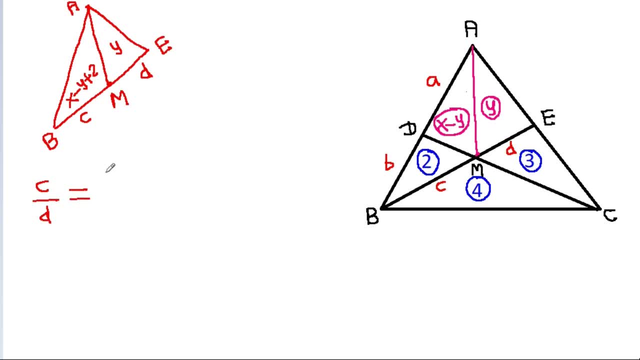 So C by D it will be equal to X minus Y plus 2 by Y. And also we have BE and C, And this point is M, and BM is C, EM is D and this area it is 4 and this area it is 3.. 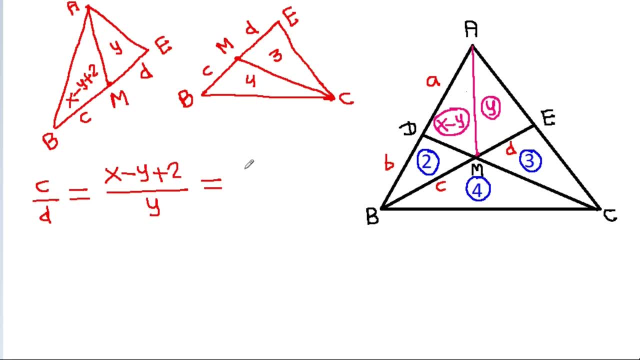 So C by D it will be also equal to 4 by 3.. And from this equation, if we cross multiply, then 3 times X minus Y plus 2, it will be equal to 4 times Y, And it is 3X minus 3Y plus 6 is equal to 4Y. 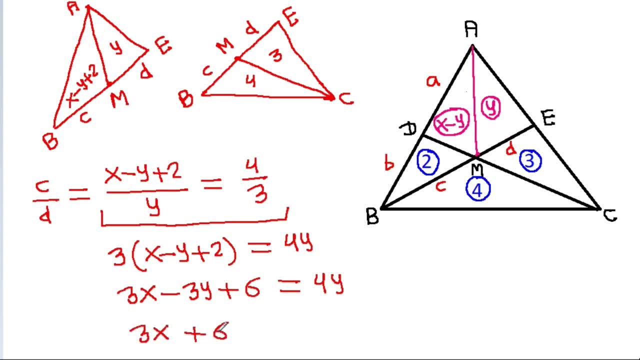 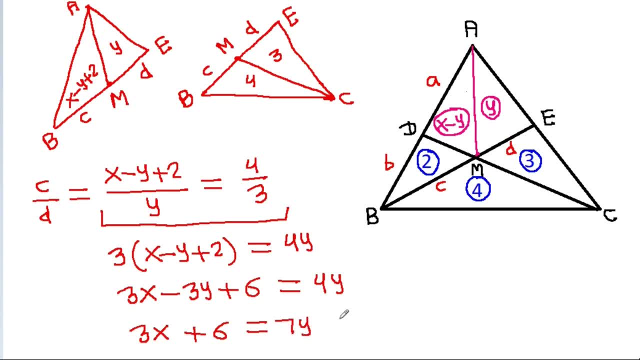 It will be equal to 4Y minus 3Y will be 7Y. It will be equal to 4Y minus 3Y will be 7Y. That means Y is equal to 3X minus 6 by 7.. 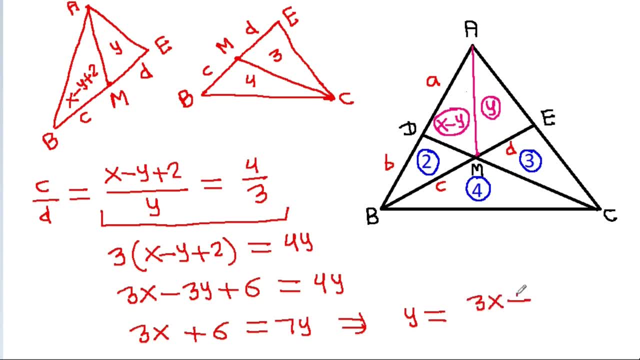 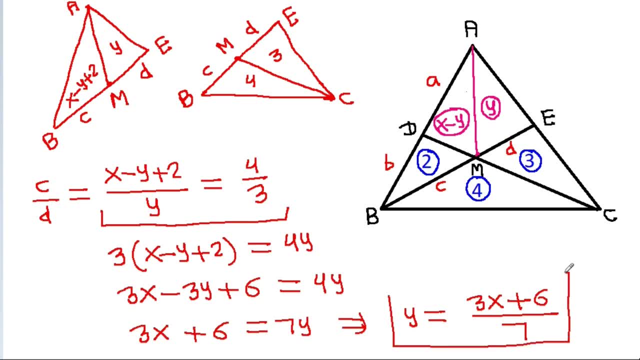 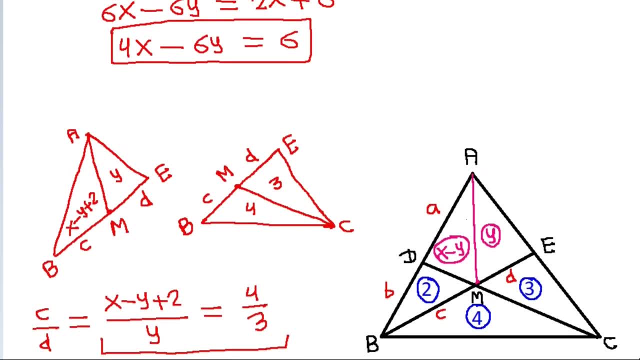 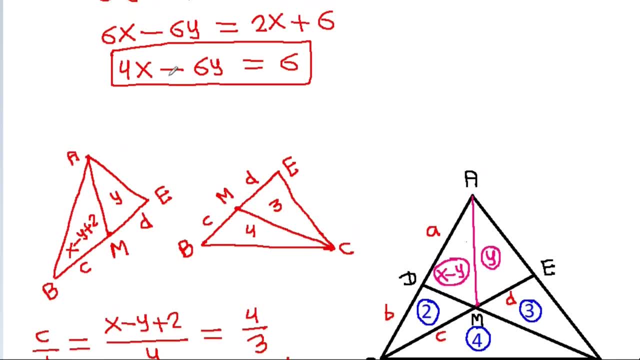 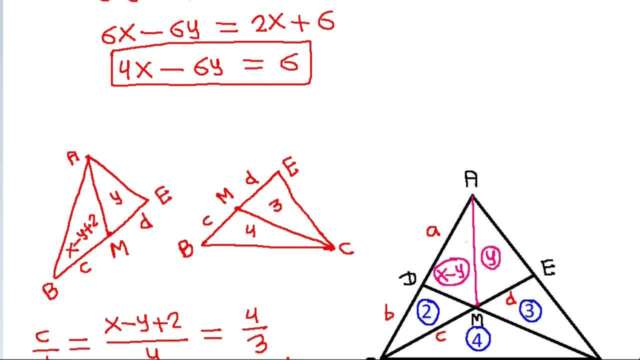 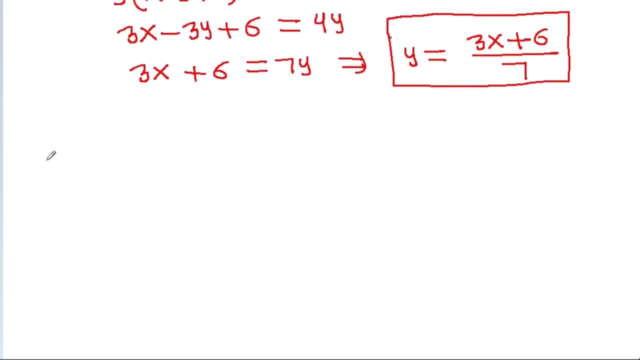 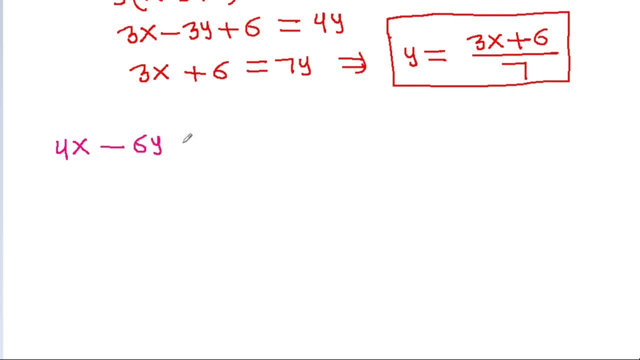 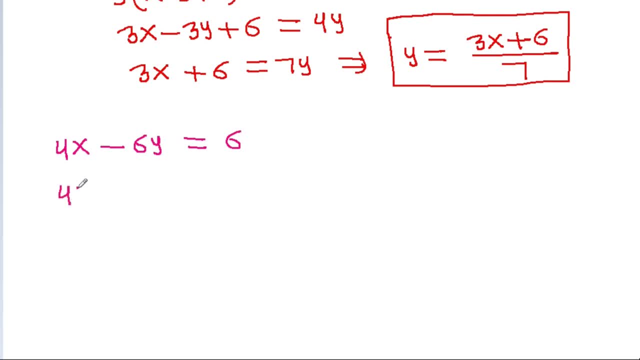 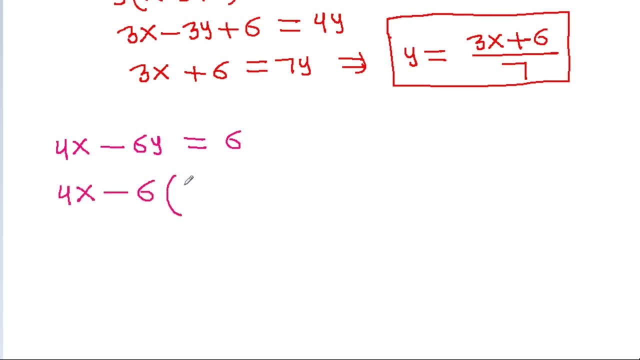 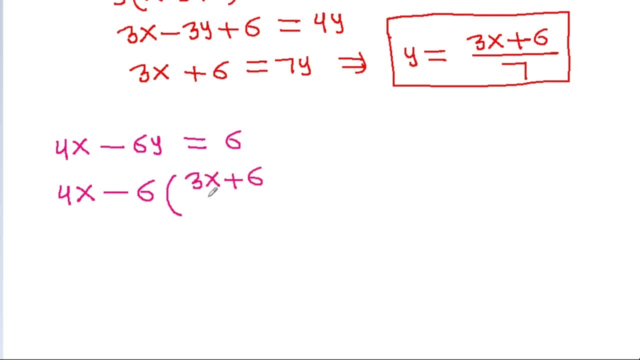 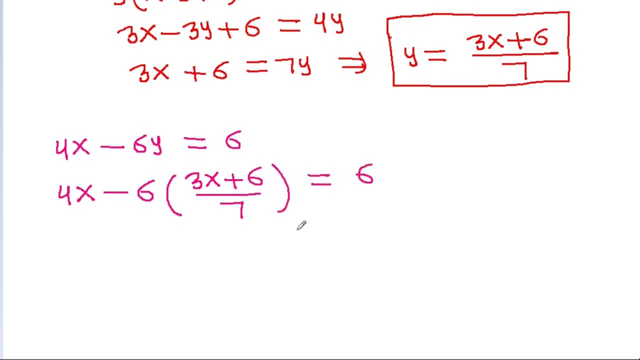 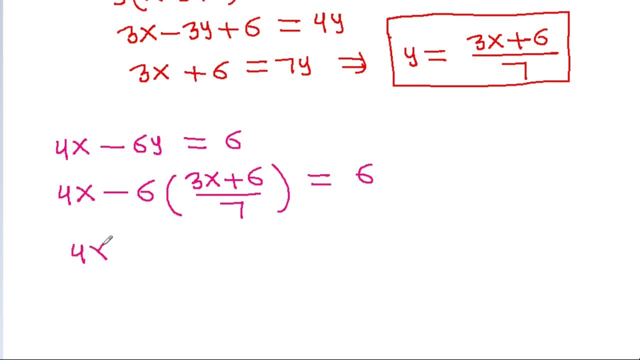 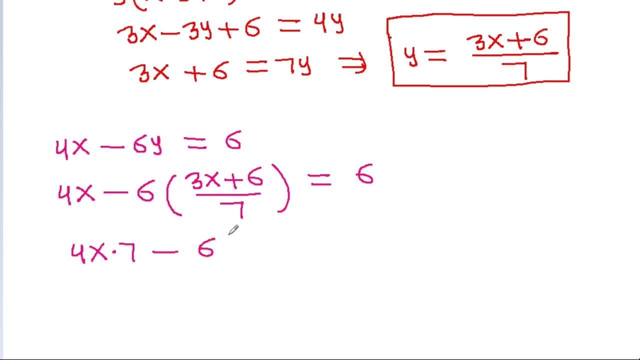 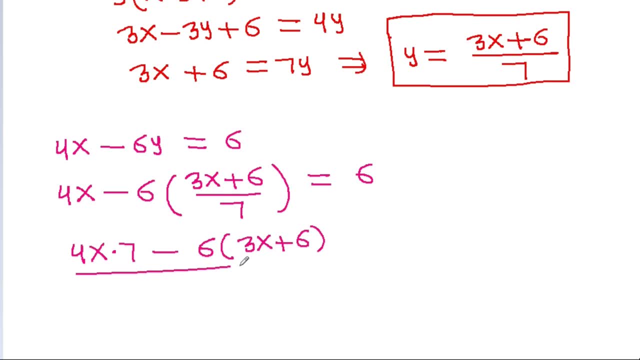 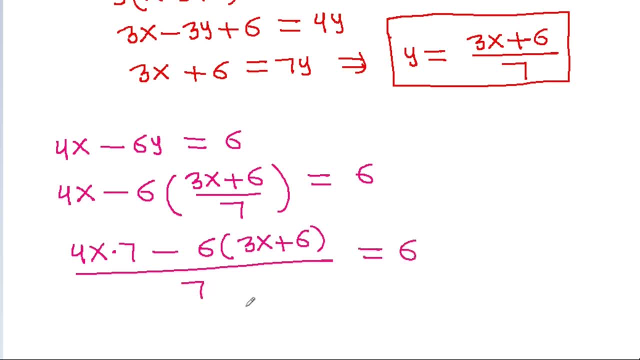 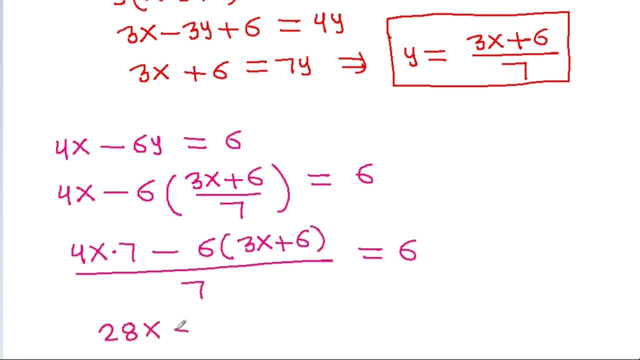 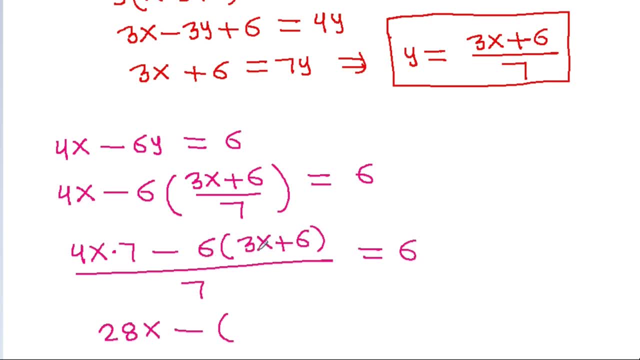 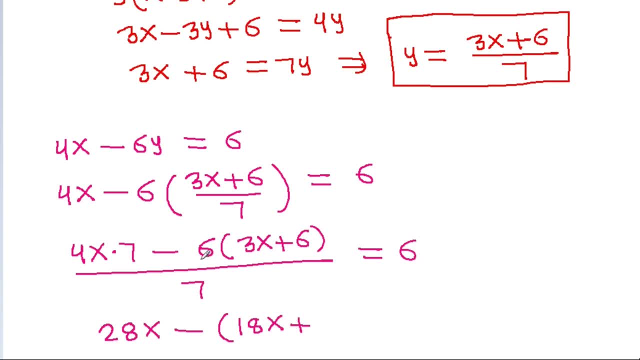 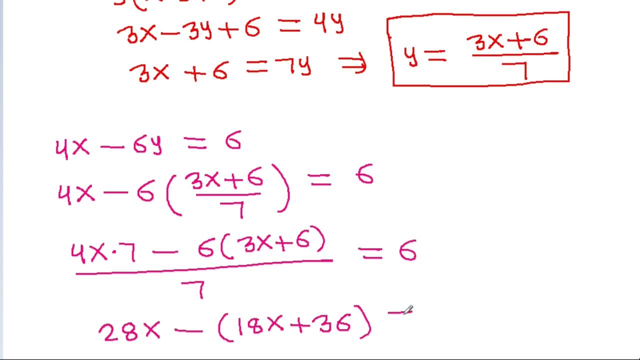 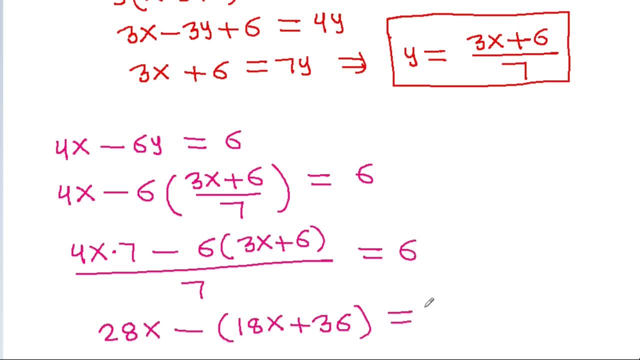 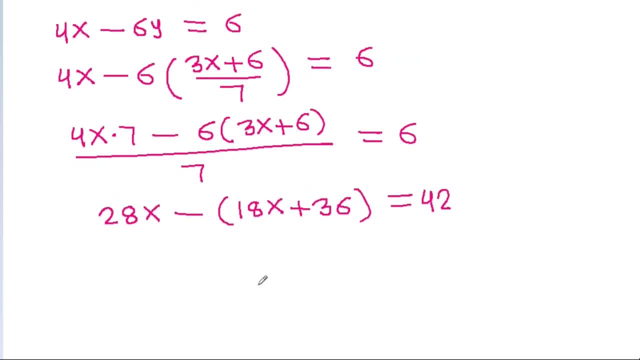 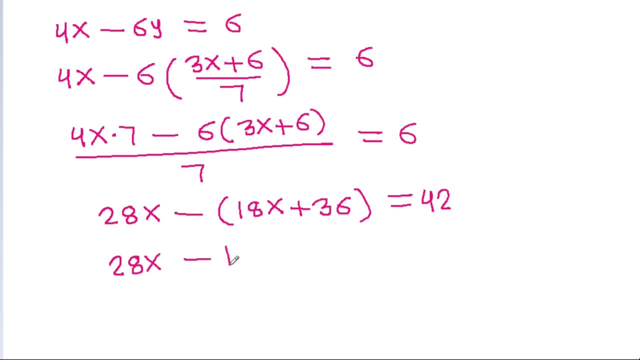 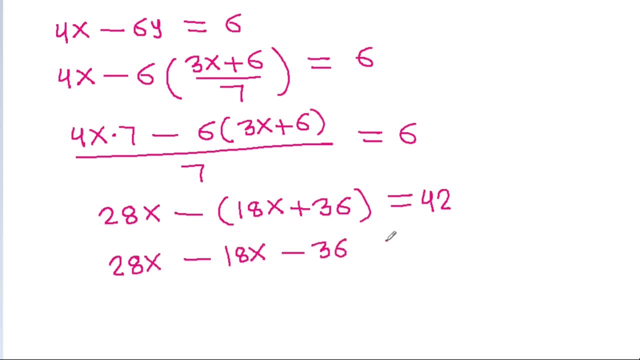 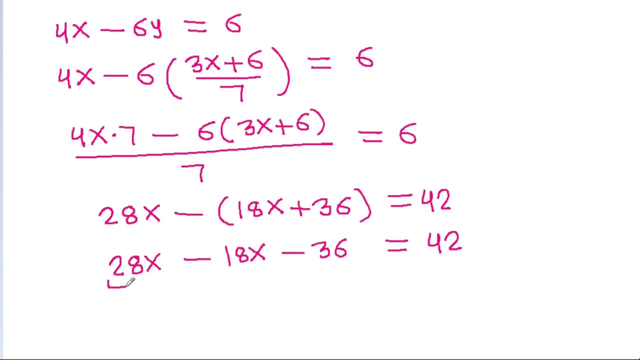 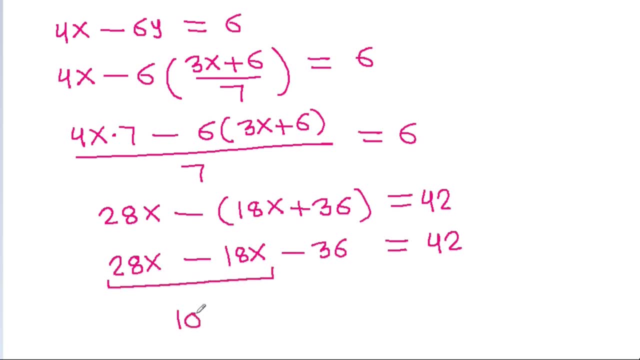 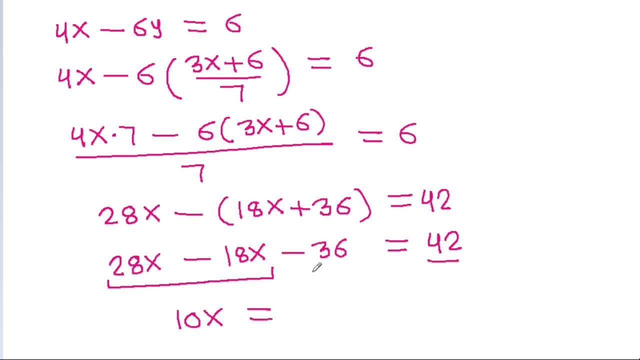 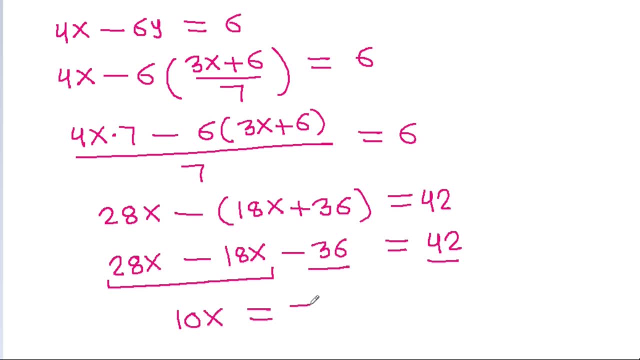 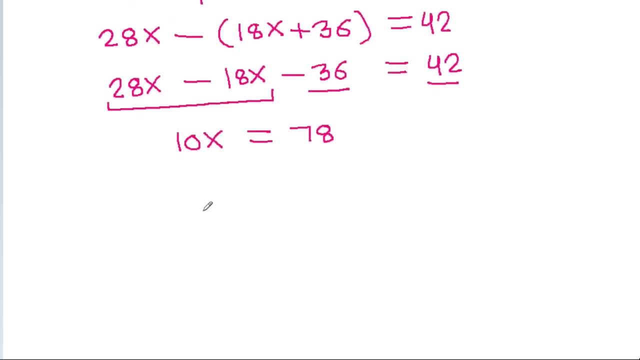 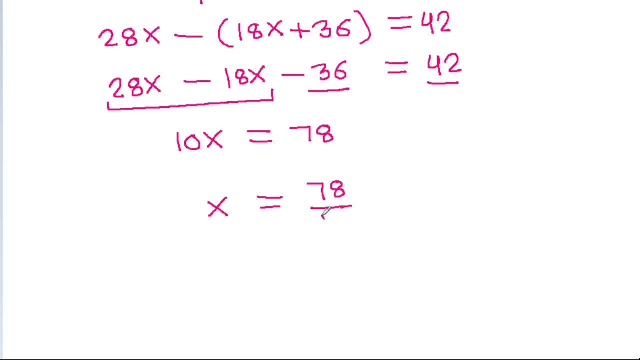 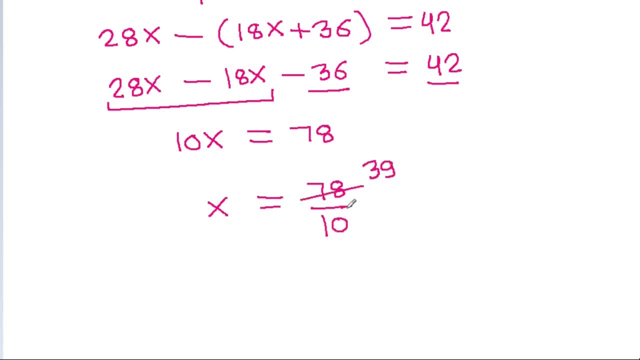